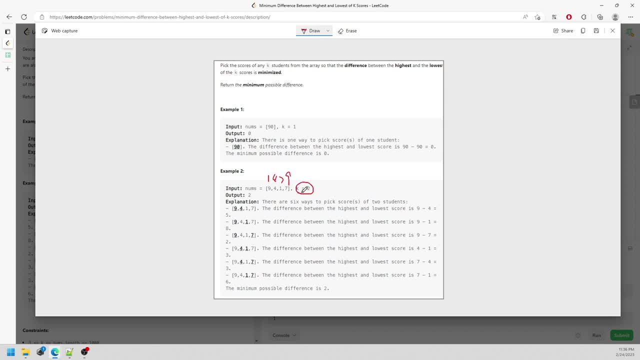 right. so I'm gonna try this based on the K right because if I have a, if I have a, the small window which is going to be the case size window, I know my left, my left most is gonna be the smallest, my right most is gonna be largest and just. 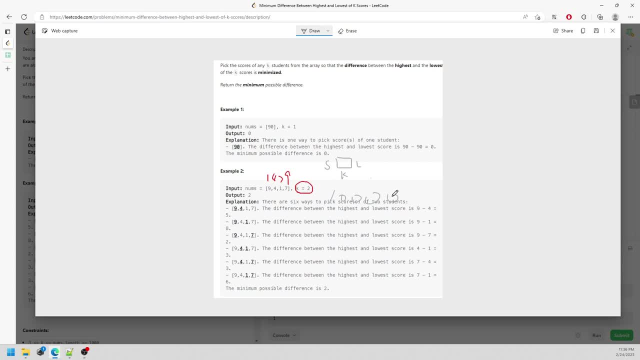 imagine I, this array is like ten thousand, right, it's like ten thousand value and your K is like what ten right? you definitely need to know these two value only right, you don't care about, you don't care about the middle. but when you traverse on the next iteration, you need to, you need to use the. 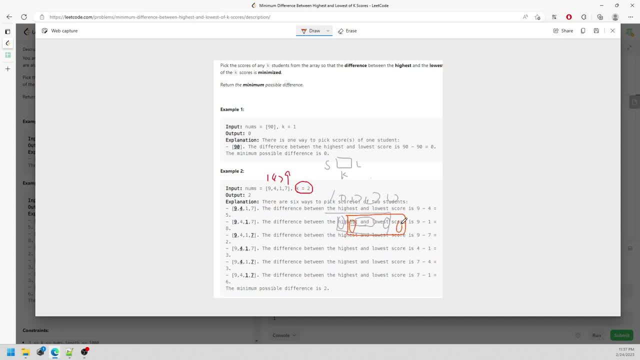 this value with, with your, you know, the current window largest value, right, so this is how it is right. you want, you want to make sure, you want to make sure the current window for the size of K windows, the largest one minus the minimum, the smallest one, is a solution. so, again, the K go to 2i. so this is the 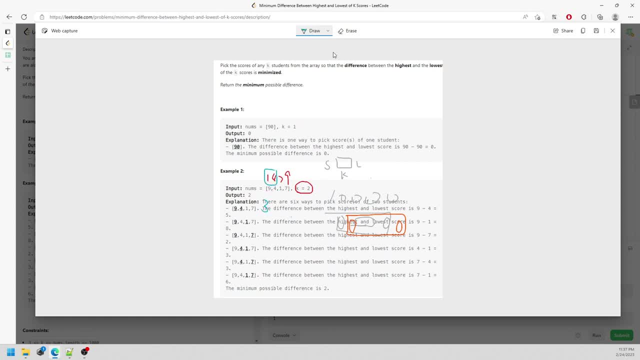 size of 2 right 4 minus 1 is actually 3, right another one, this one, 4 minus 7. okay, you know 3, and this is what the size of 2, 9 minus 7 is going to be 2. so the answer is 2, alright, so you, well, we know this. 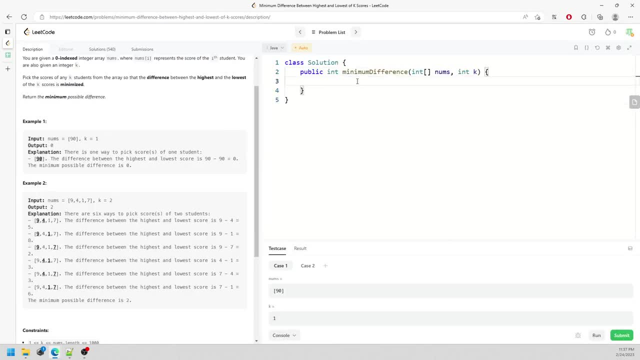 idea. right, you can stop holding. so what you have to do is, while you just sort the rate for the norms and also you need the return value, it's gonna be what I'm I'm making the value for the, for the largest you know, and I'm going to just 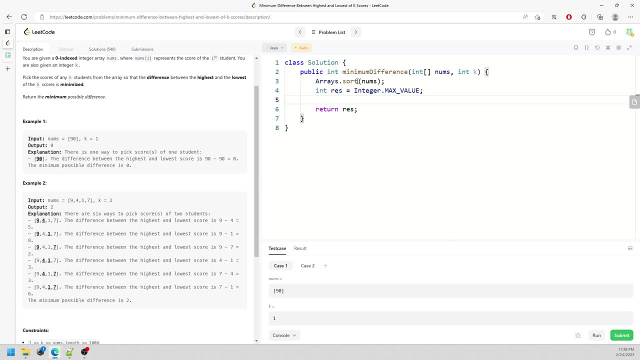 keep mean minimum for the you know traversal. so I'm going to start in from what. so it's it's not starting from K because case the starting value is starting from 1 right and then a race is based on in the 0, so you have to say K. 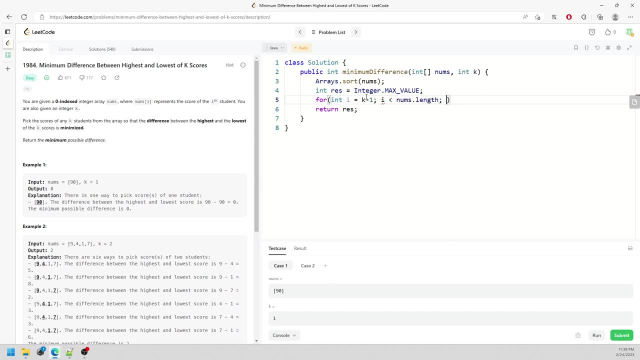 minus 1, I less than num, stop length, and I plus plus, and then result is going to be math on mean right. we take the mean for the turn turn result as well as the num. say I minus num, say I minus K plus 1. so if 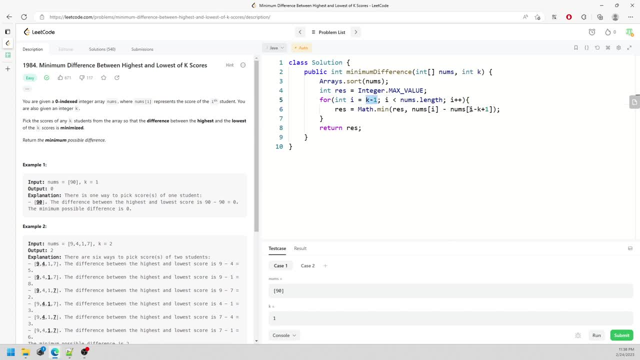 you just put a K minus up, K minus 1 inside. here you add. you add up what to 0, right, because I started from 0, right? so I mean this- this is a map, you know the case- to the part inside the window K. so let me. 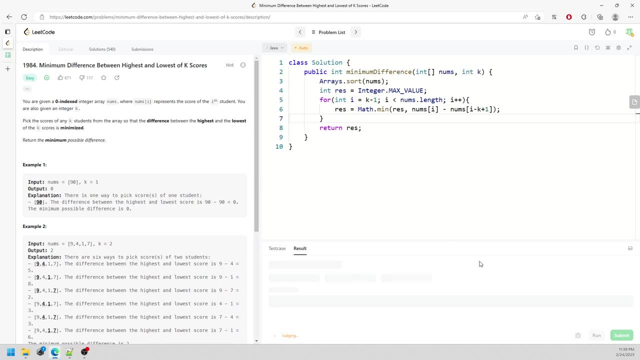 just run it and submit. so the time and space are pretty straightforward. this is what this is: a time. this is also a time time for the sorting is: and often and represent end of the nums array, and then space is constant. right, you don't need to allocate any space. 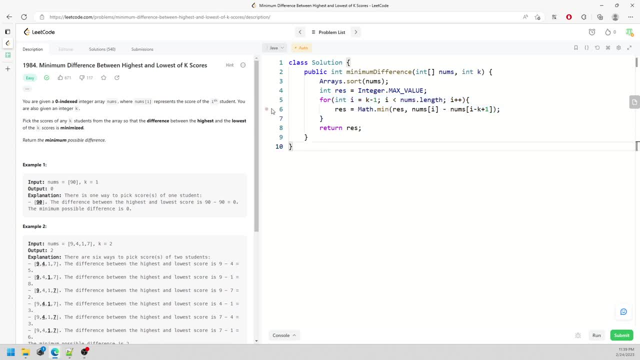 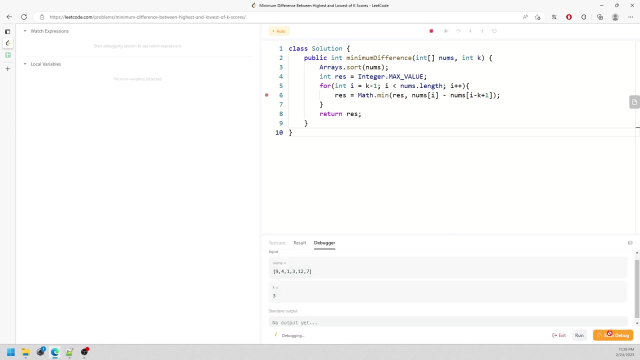 and this is all of them for the time. so this is pretty much a solution. so let me see right. so they just run the test case for this one and hopefully you get idea, and all right, cool, so just keep looking out, looking on the left window, and powers any second finish. 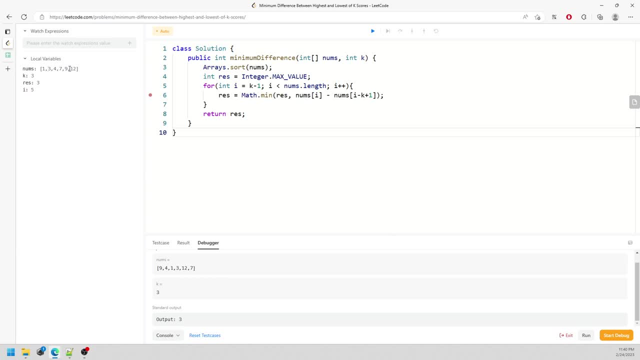 up a 3, my right, haha. yes, yes, the Гос Independent3 right, and what you have to do is why just leave a comment if there any question? actually, I wanted to take you to this is this is more doable for you to think about this? 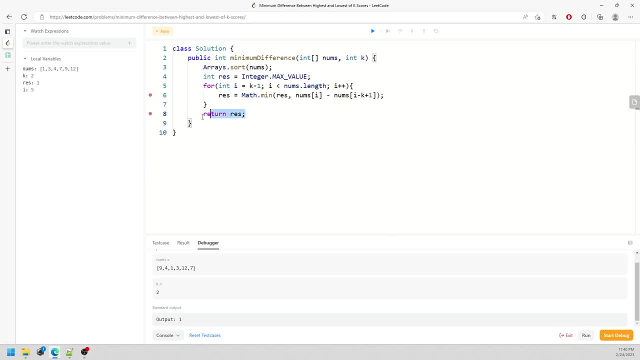 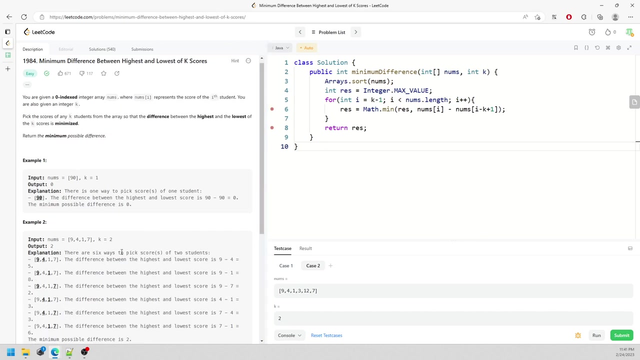 all right, I didn't. you know, I didn't pause my return value, but the answer is one right, so whatever, and if you still have a question, just leave a comment below and I subscribe if you want it. but the idea is I using the size of window K. 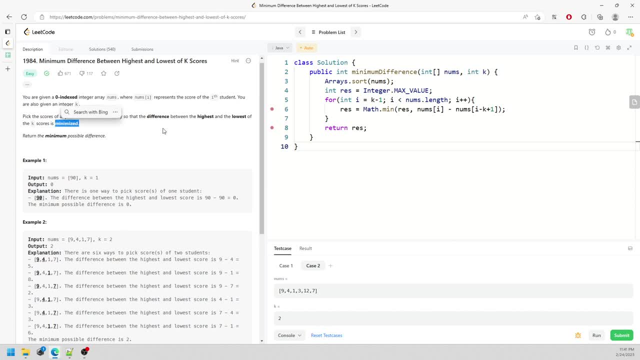 to find out the minimum value. you have right, just the left, most outside right, most minus left. most is actually your. it's actually your return value, which is the minimum, but just depending on your traversal and this will be the solution. so if you still have question, leave a comment below. subscribe if you.